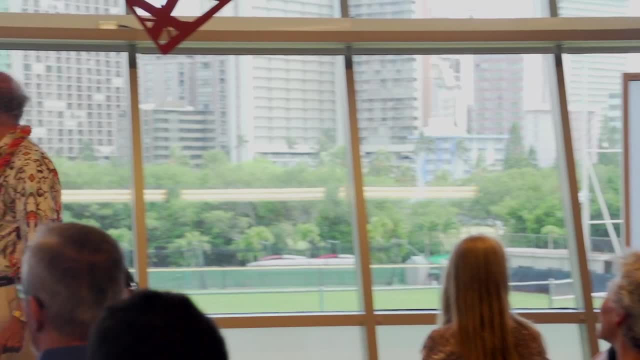 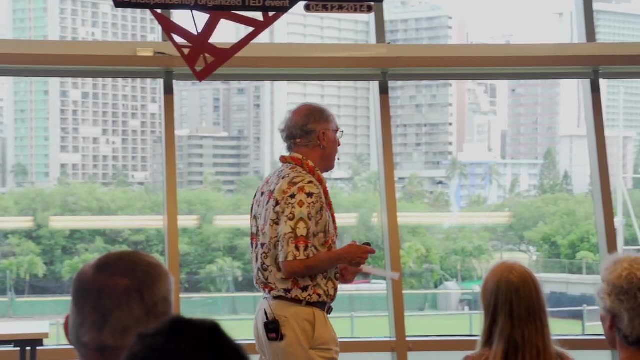 it's sort of why I believe in miracles. behind that name is a 1.25 million dollar grant that we got for the work that I've been doing for 30 years. the other one, home of P4C Hawaii. I'm going to be using this expression, P4C- any of 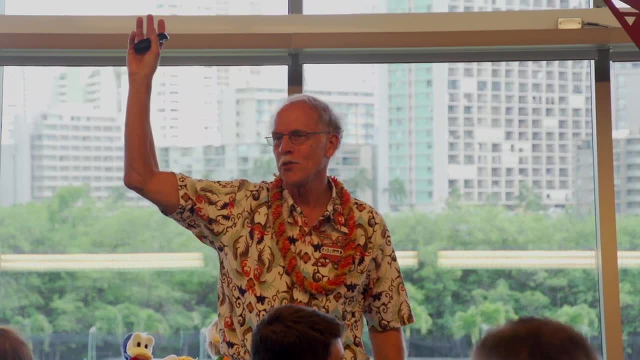 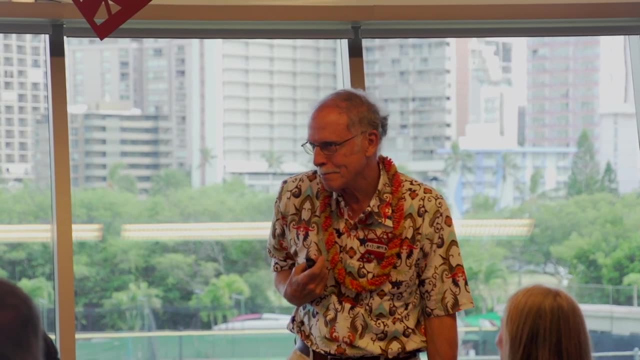 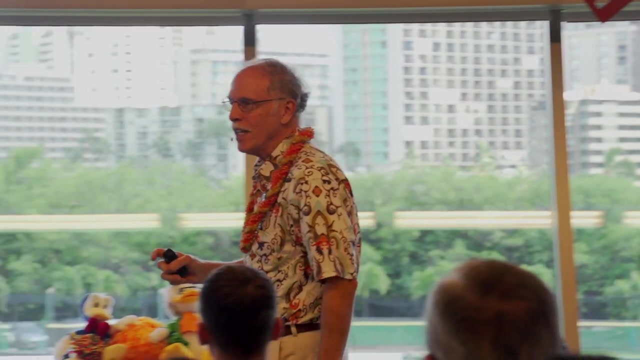 you folks heard that expression. let's see, okay, good, there are a few folks out there, all right. so the P stands for philosophy, or as we put it, with the kids below. so, and the other one stands for C, or children, and so you're going to be. 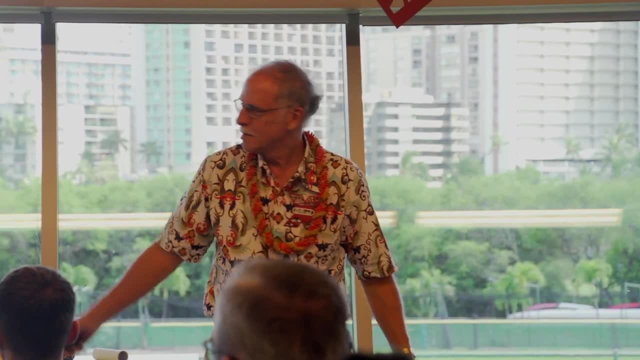 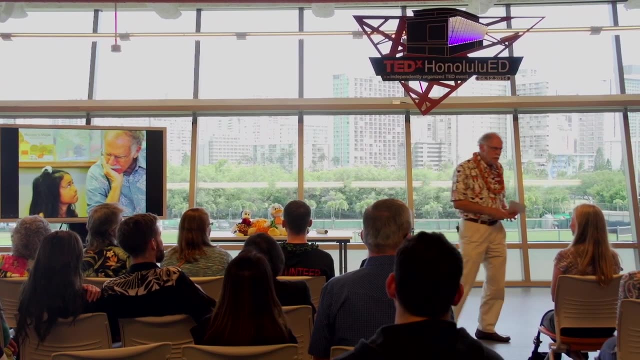 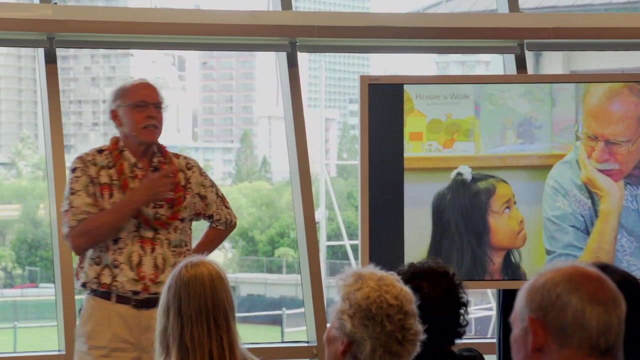 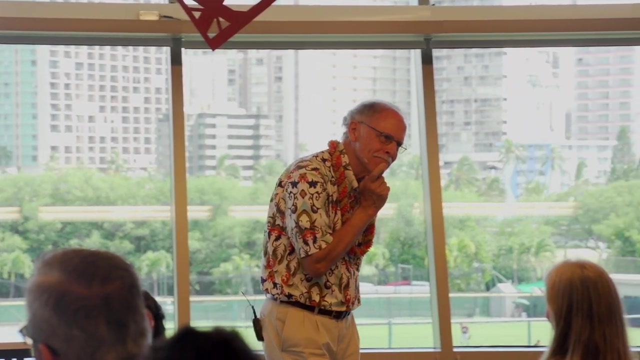 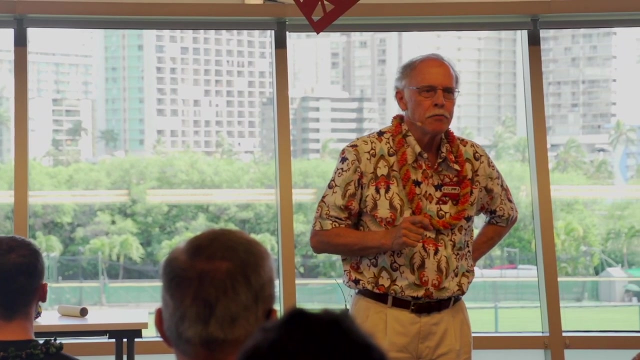 hearing P4C quite a bit. now my other slide: oh, I brought it back. okay, this, I love this. I really love this, and my title for this is one of my subtitles for this is: it's a wonder moment. for this is it's a wonder moment. 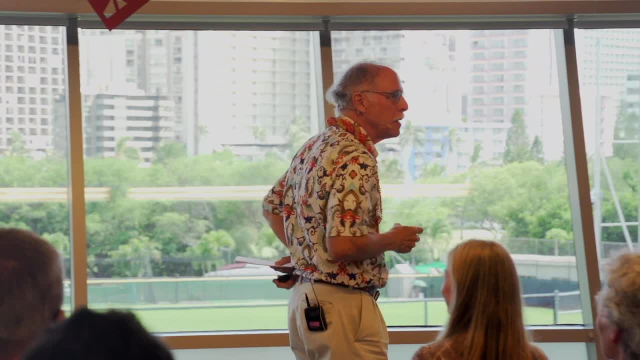 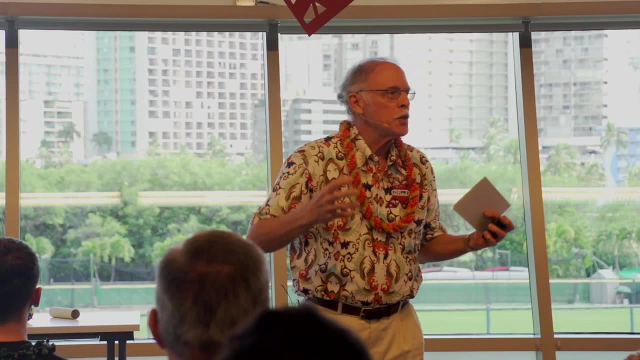 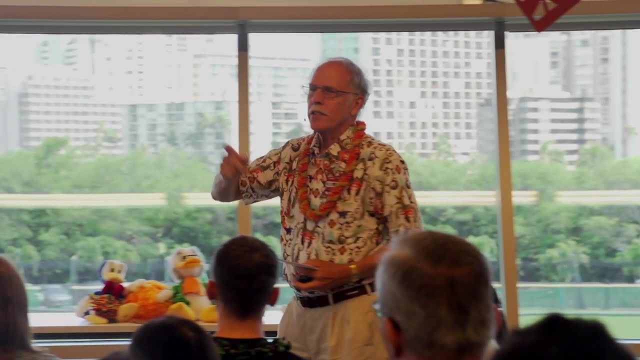 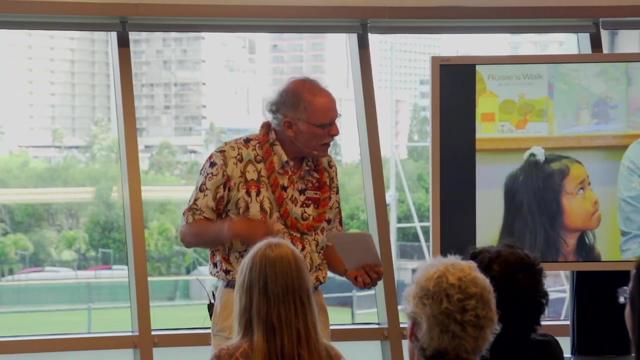 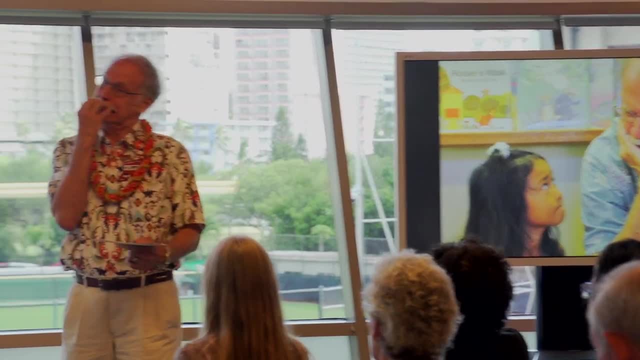 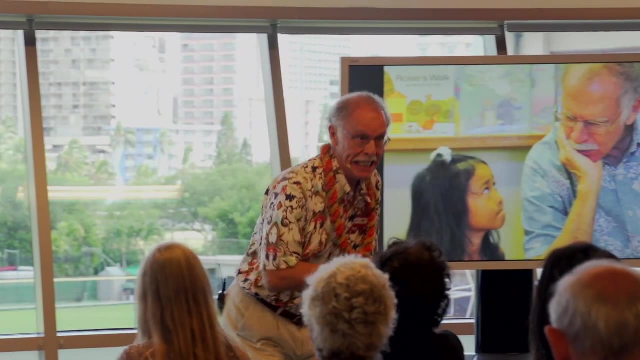 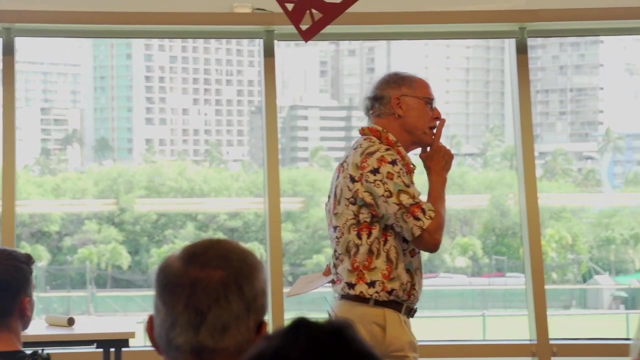 after draft after draft: Here's this fantastic opportunity. So last night when I fell asleep, I was on draft number 19.. Yeah, and I had some very good coaching, thank goodness. So it was draft number 19.. I thought it still doesn't work. It's still not there, And I 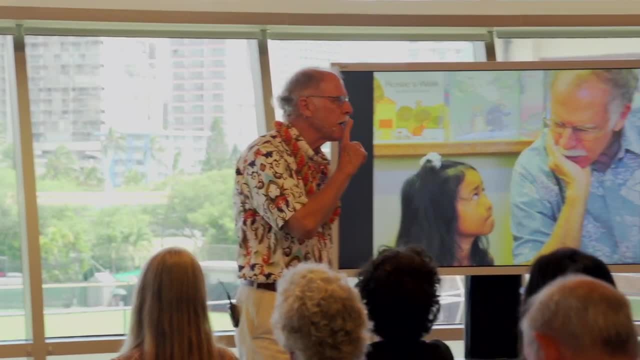 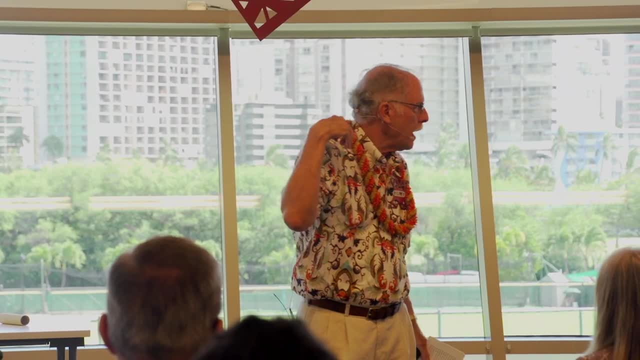 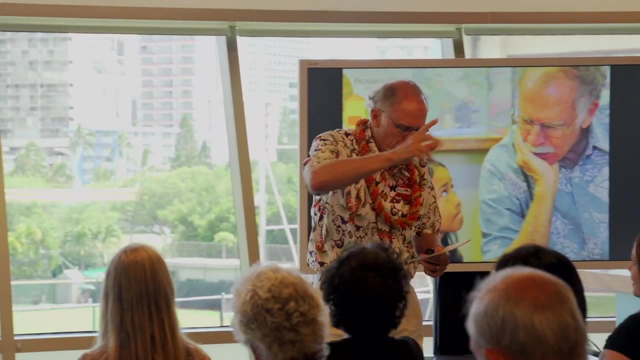 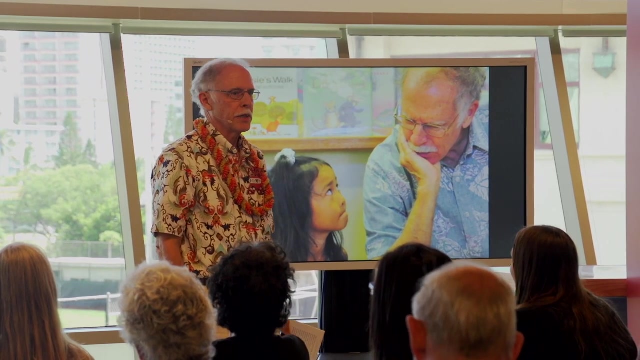 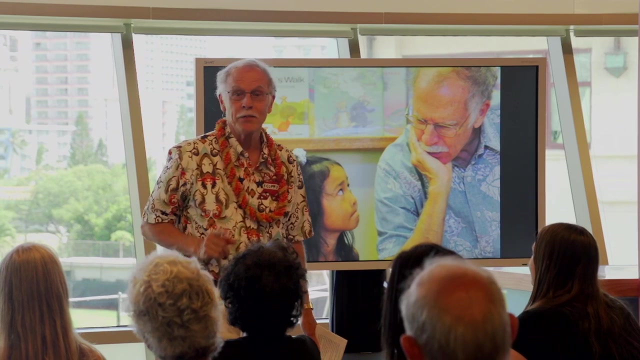 up this morning I thought, okay, what am I gonna do? what am I gonna say? and first that slide came to mind and then I all of a sudden in my mind I hear this one's for Gabby, this one's for Gabby. and if you know Israel and you know the facing, 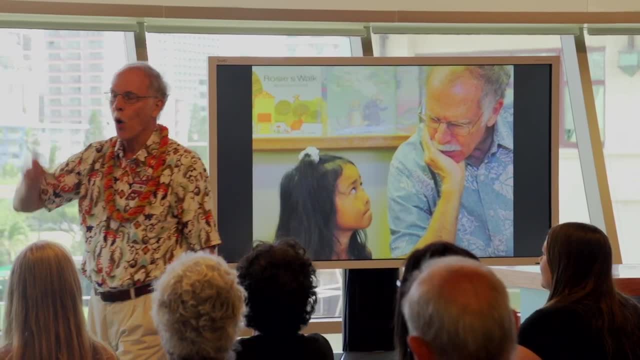 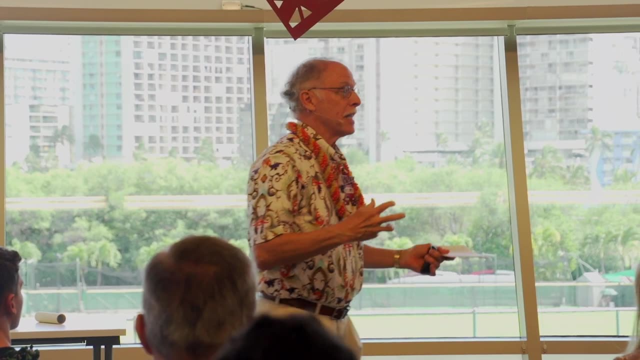 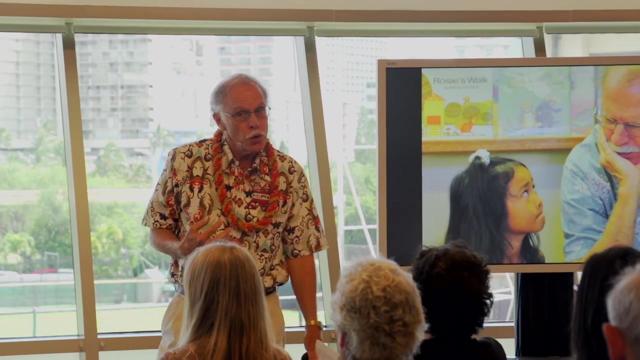 future. that's the way over the rainbow and it's a wonderful world starts out, and it still gives me chicken skin every time I hear it. this one's for Gabby, and for folks who don't know who Gabby is, I'm figuring it's Gabby Pahinui. it's. 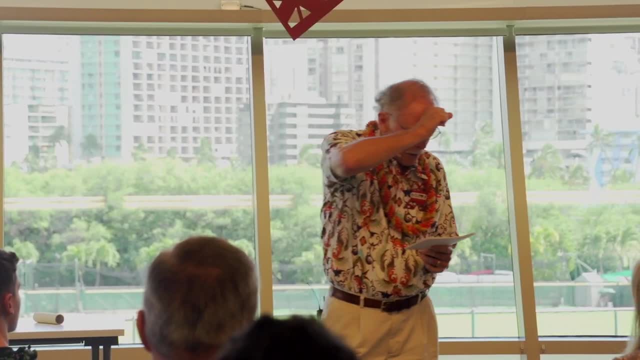 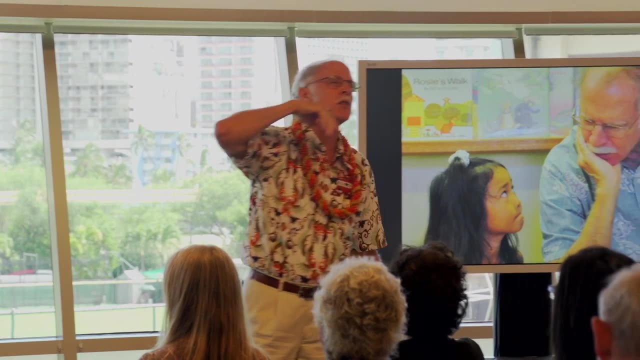 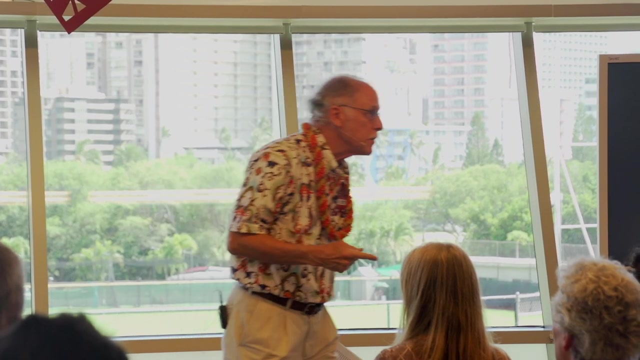 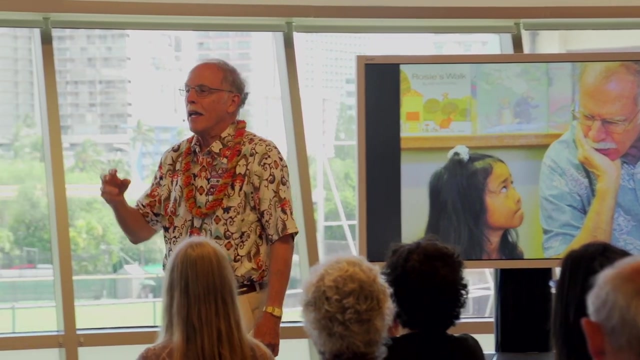 Gabby Pahinui. and then I hear: and I've got this. I thought if I had asked you guys sooner you maybe could have played it, because there's this place where it says: and the somewhere over the rainbow, the dreams that you dare to dream really do come true. and then I hear babies cry. 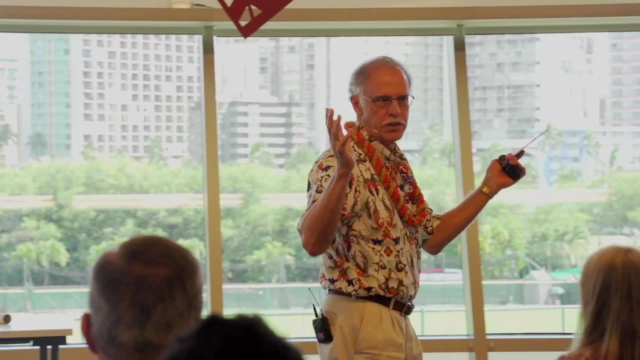 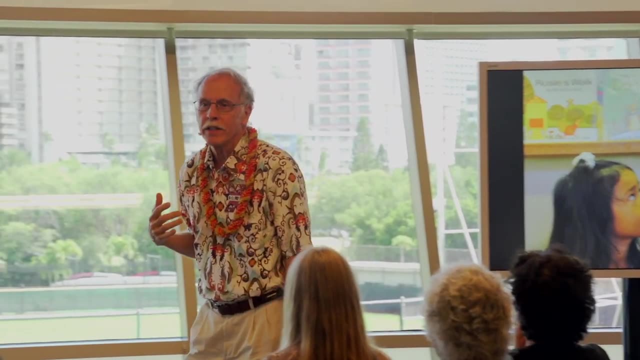 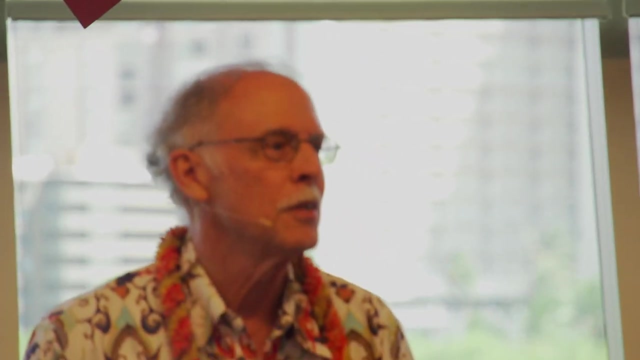 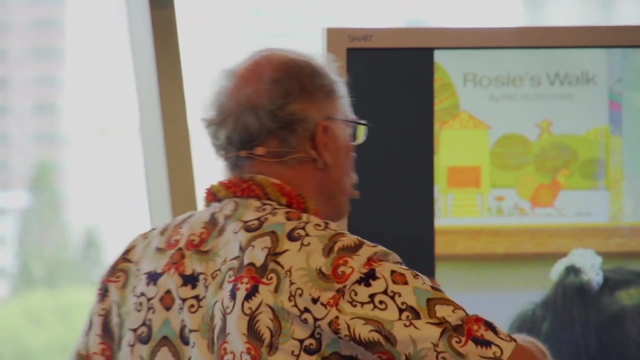 and I'm hearing this, and they couldn't last it more than a couple of seconds, but it was just like that. I watched them grow. they'll learn much more than I'll ever know and I think to myself: what a wonderful world. so then I'm thinking about, and I've named her Tiana, and I'm thinking about the two of us too. 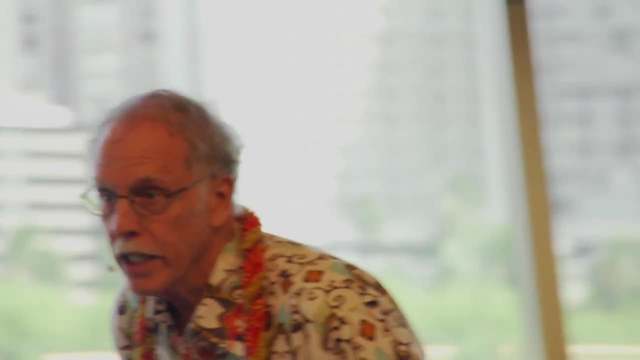 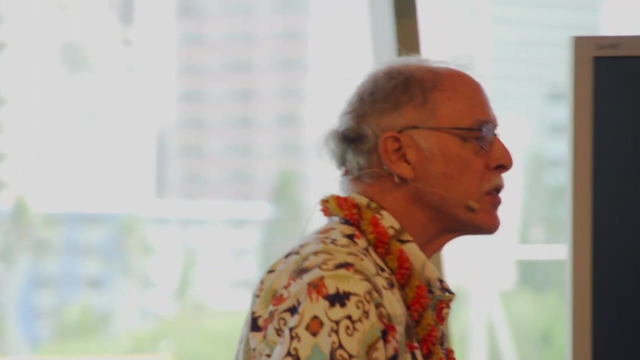 there and we're both it. we didn't know the picture was taken and we're both deep in, hmm, and I started thinking about what a mess the world's in, what an awful mess. and you know, you look at that time zone in the middle of the universe, at this time of the universe, and this is when things will actually really shift. then you look at that time zone in the universe and you realize it's not there yet and I started thinking about what a mess the world's in, what an awful mess. and you know. you look at the time zone and a bunch of people are in there. 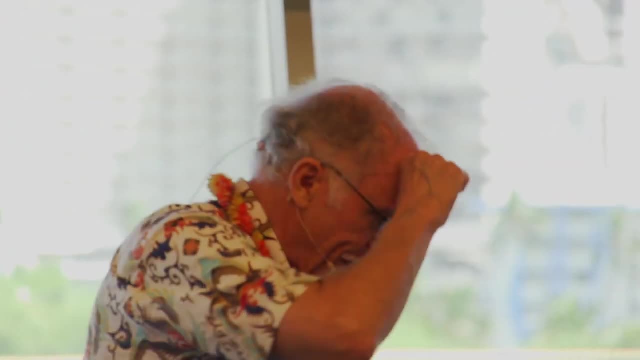 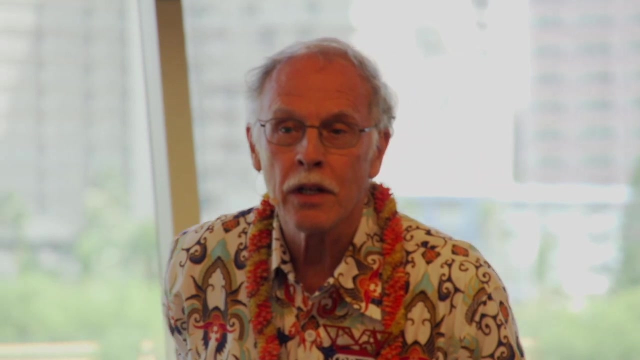 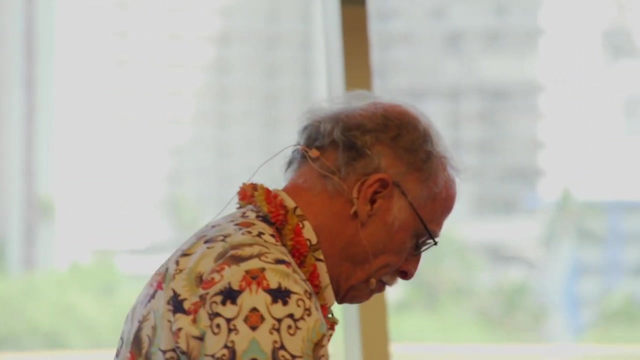 lines, but you hear about the things that are not working and I think about her and as I look into her eyes, I'm thinking: but you know what, Tiana, it's going to be okay. it's going to be okay because we're going to figure this out. 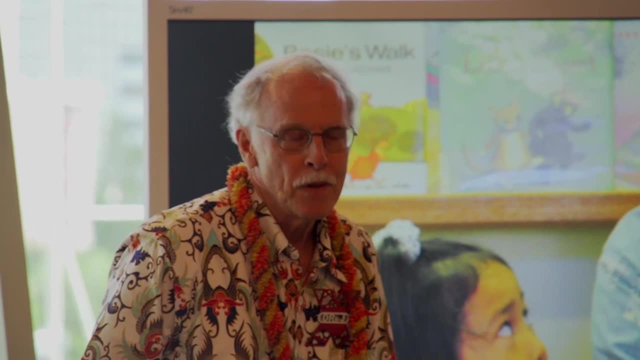 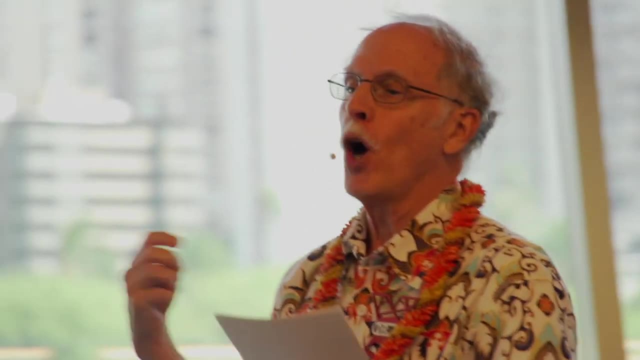 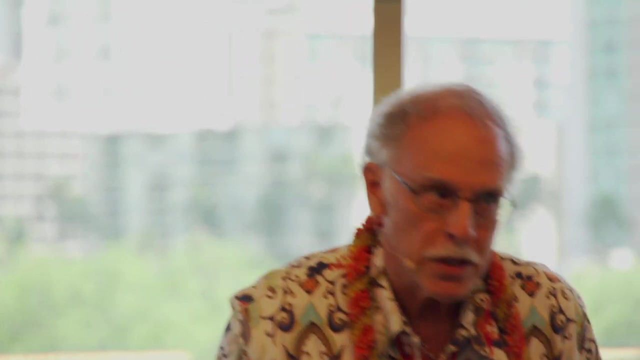 together the work that I get to do with young children. every time I come away I am so filled with optimism and hope, and when I say we're going to figure this out together, I mean not me. part of my message today is how desperately we need those very young children. 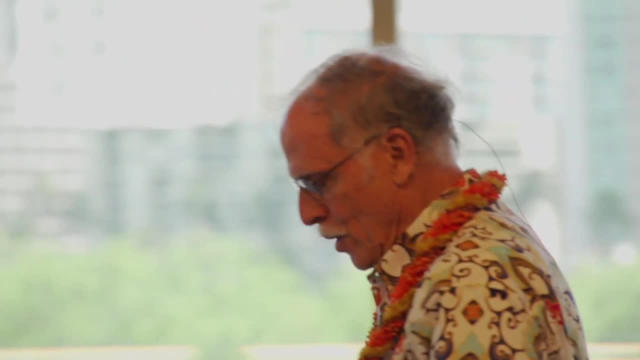 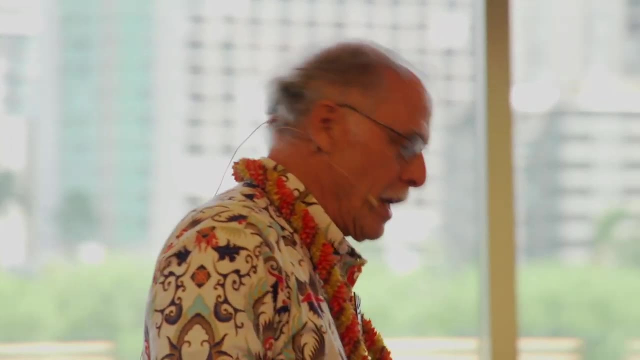 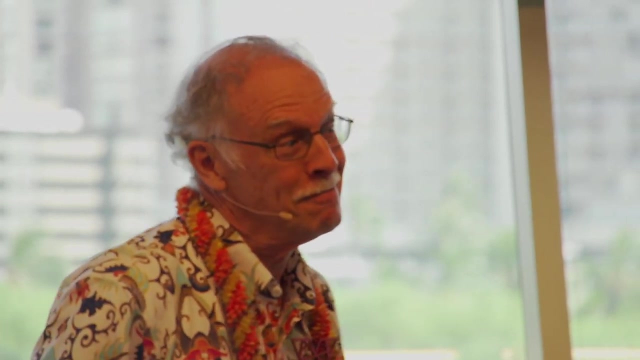 and those very young minds. so then I finally hear this like, well, I'm going to do that again. so then I hear this thing that says: don't don't do that, don't be nervous, because this one's for the kids. so I'm going to try not to be nervous. 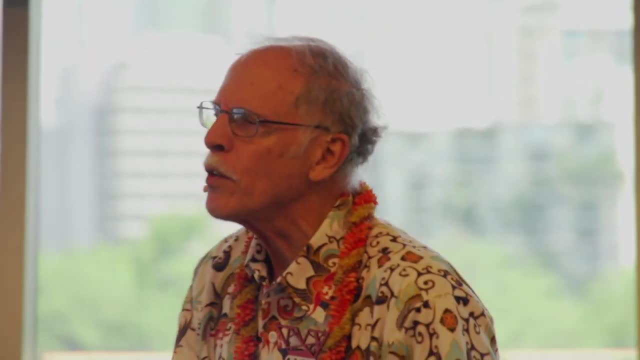 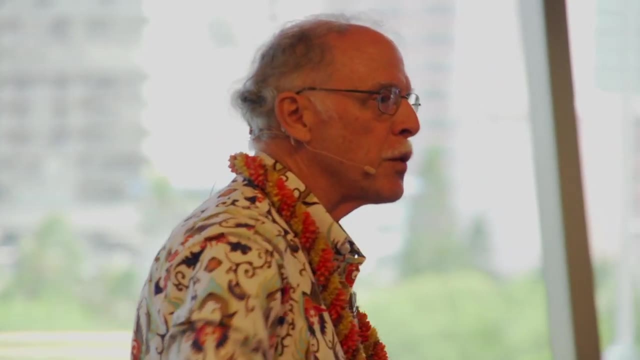 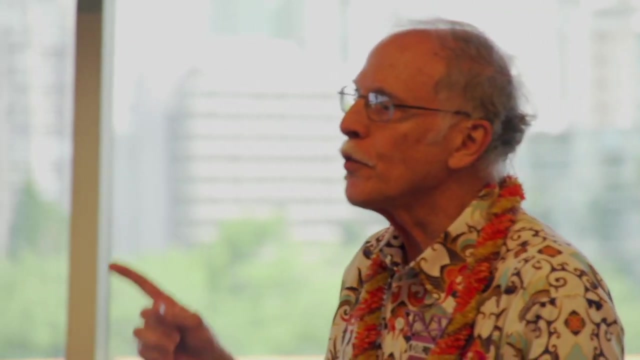 now I have a question for you guys. oh, I know. the other thing is that she asked me: how are you going to do that? and I said, okay, I'm going to share with you adults here today all that I've learned from you folks about doing P4C. 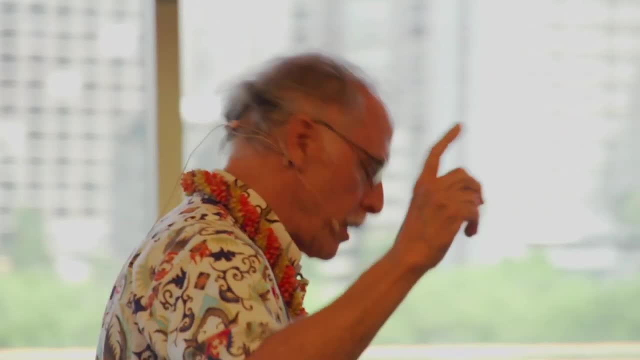 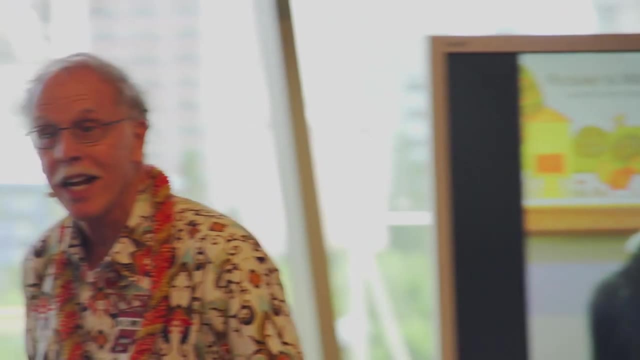 together and I'm going to share with you folks, and I'm going to do that to the best of my ability by using your voices, not mine. I don't want to tell you about it. I want to use their voices and I told her. you know what? 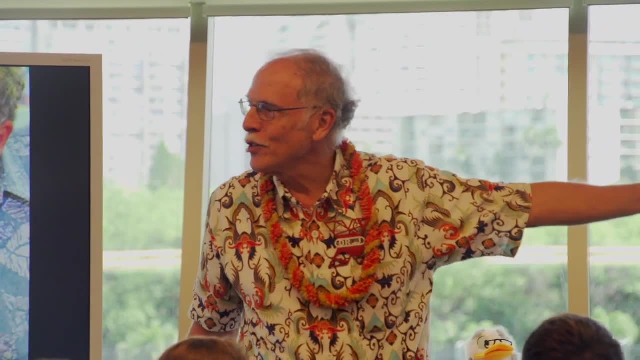 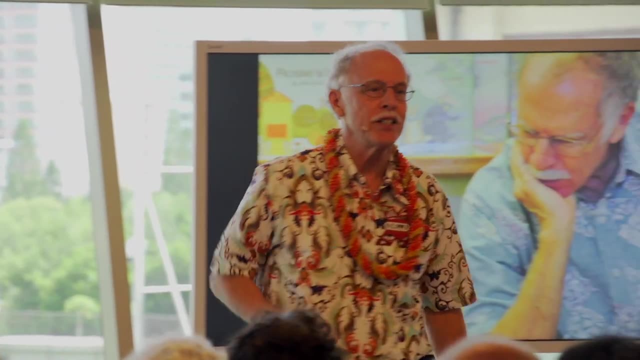 they're going to take a video and when we're done we'll sit down together and watch and you can tell me how good a job I did. okay, now question how many of you folks were a child at one point in your life? right on, I've never had a hand. 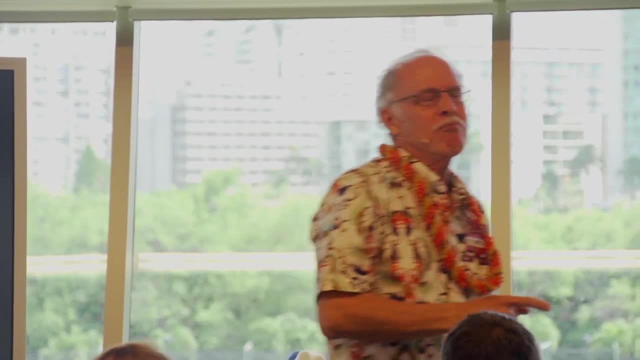 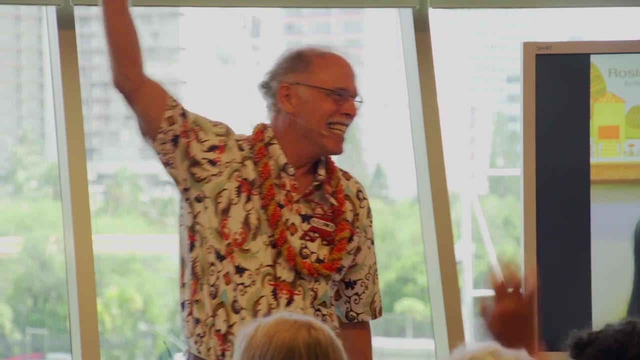 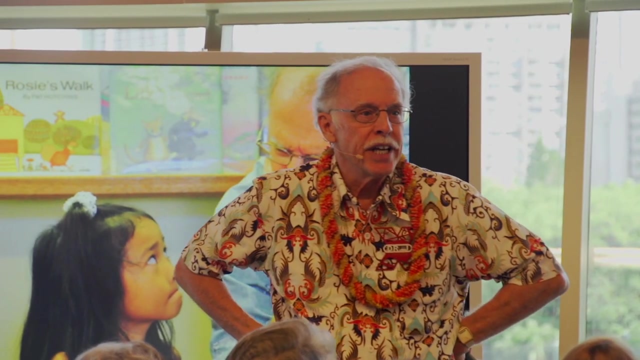 not go up. it's very encouraging, and now maybe a tougher one. how many of you folks would still say: you got a child in there somewhere still, oh, see, see. so how many of you guys wondered as a child: oh, look at that, you should turn around and have a look. 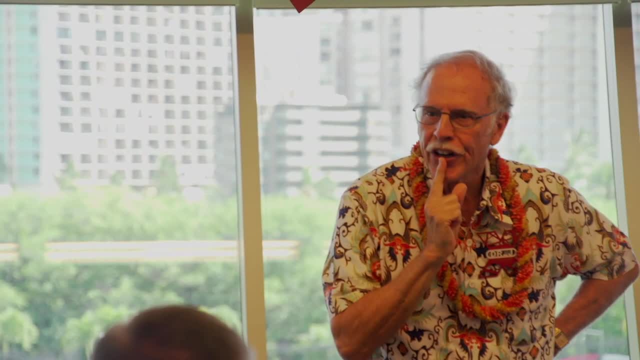 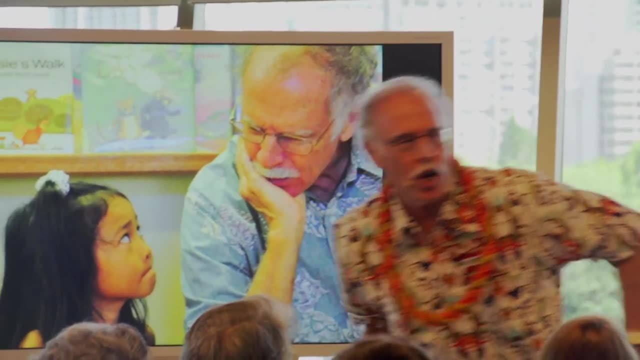 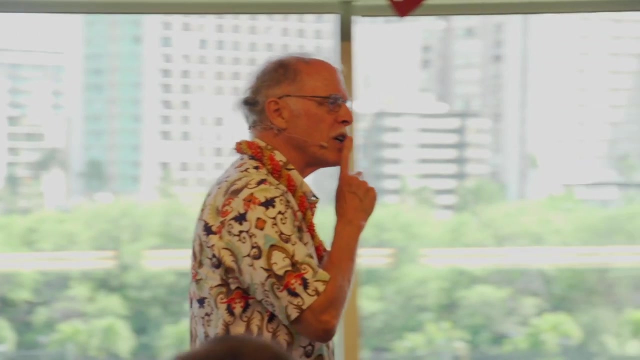 you know that's very encouraging. how many of you still wonder, okay, see. well, I want to introduce the idea of two kinds of wonder. I want to call it deep, deep, deep wonder, and the other kind of wonder I want to call practical wonder, like: what am I going to fix for dinner? 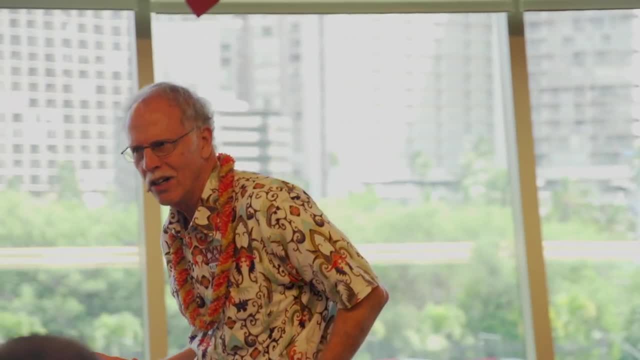 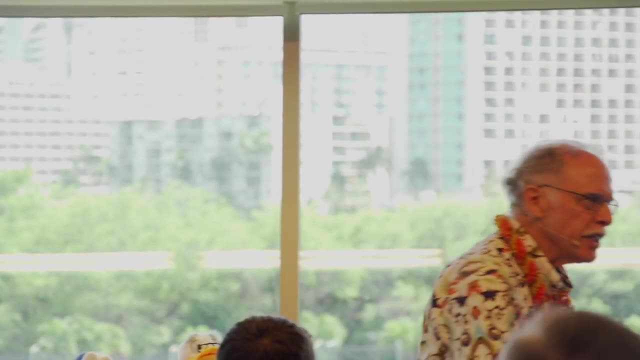 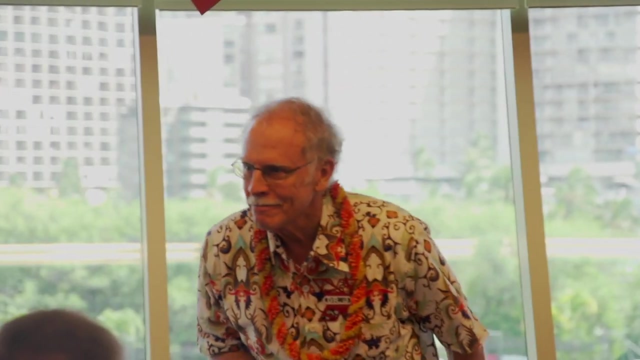 you know why isn't my boyfriend called, or you know all that kind of stuff, and insert this. the what do you wonder question is a great question. it's a great question, great conversation starter. how many of you are around? young children, yeah, okay, ask them. what do you wonder about? 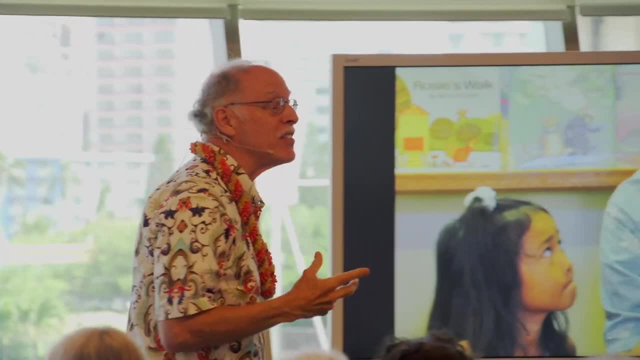 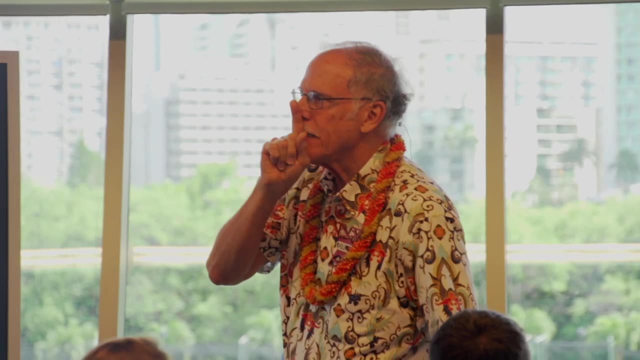 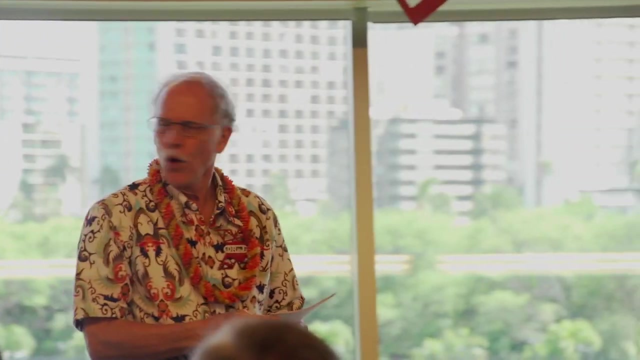 and fasten your seatbelts, because it's amazing the kinds of things that they'll have to say. so, and I don't want to forget to say this, one of the secrets: if it's a secret: wow, we're almost half done. boy, it's really flying. 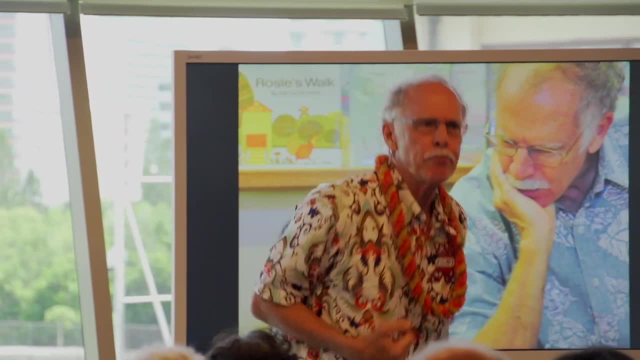 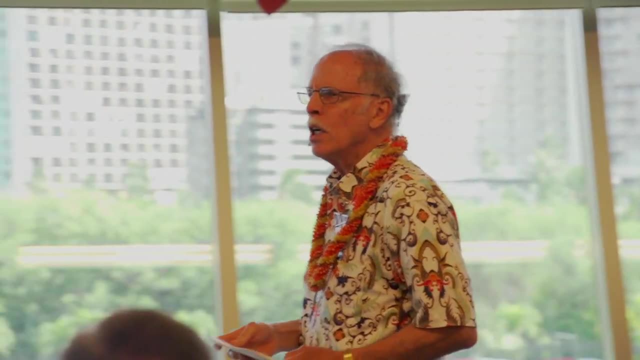 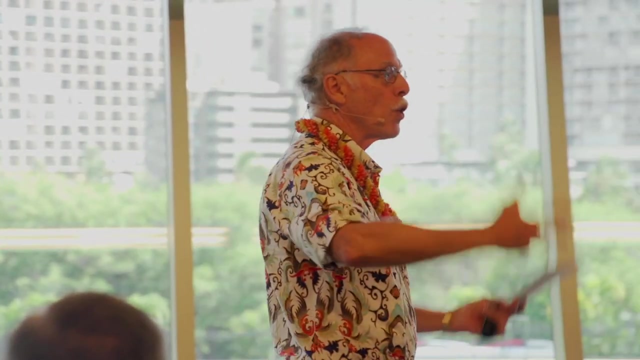 okay, but you know, part of my work is not being in a rush. at the heart of everything we do we're not in a rush and so I figure one of the things I'm really good at is ending on time, because in the work that I do, 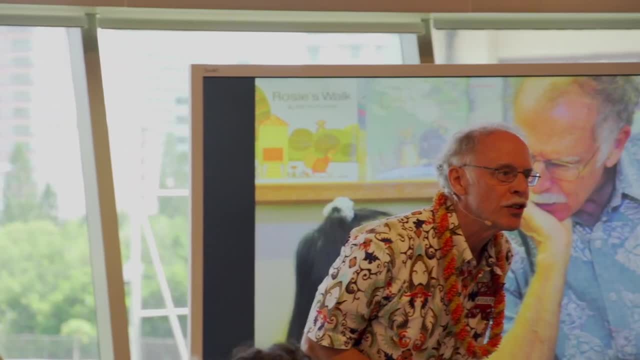 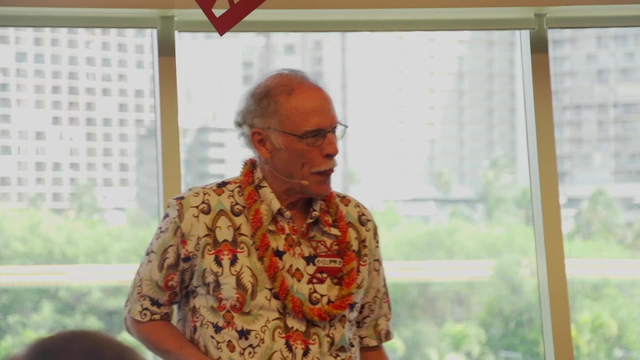 and the kids that I work with. we come up with. I call them magic words, and one of the magic words is: it is, it is, it is stands for. I don't understand and I want to empower everybody, and I want to empower everybody, every kid in the universe. 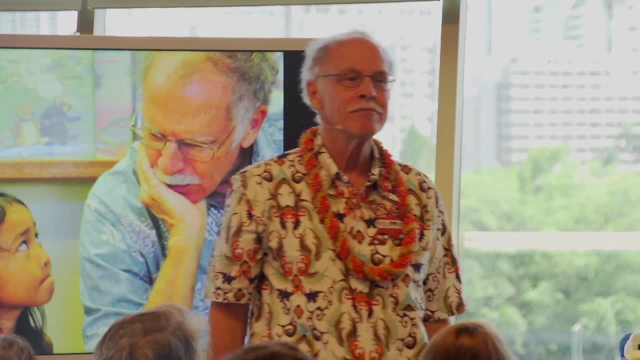 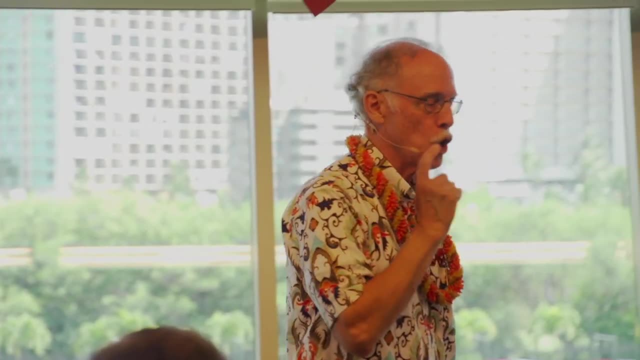 when they're in a situation in a school or whatever, to say it is because I hate to say I don't understand, I wouldn't do this, I don't understand. it sounds so mean. one of our magic words is oot. do you want to say that? 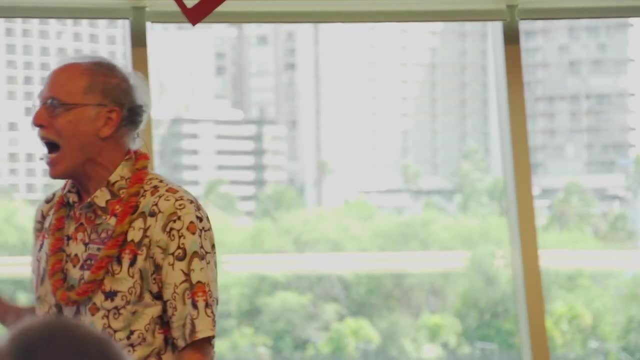 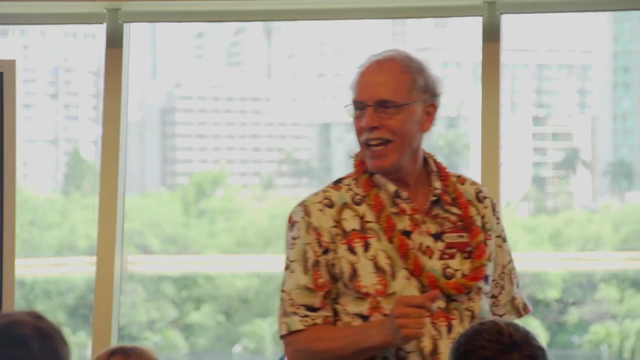 oot, oot, oot stands for out of time. so when she holds up the sign that says two minutes, I'm just going to say a oot, I've got two minutes, and when the two minutes is up, I'm done and it might be mid-sentence. 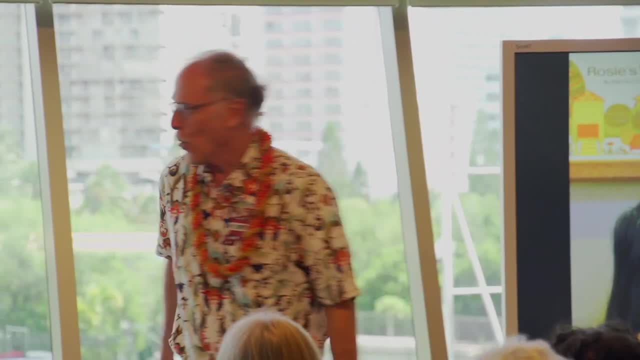 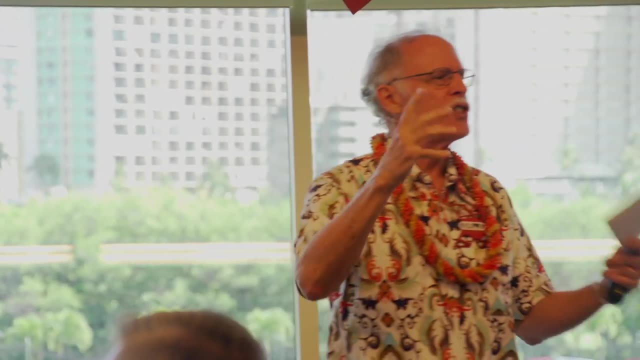 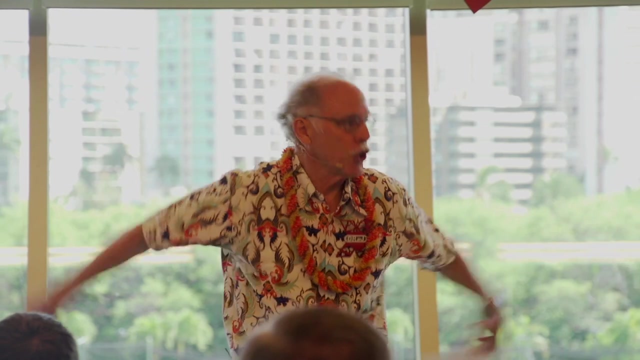 okay. so I want to tell you just a little bit. maybe I'm only going to get in one story, but that's okay, because stories tell an enormous amount. what we do in P4C- not in rows- we always make a circle, we always jeez. 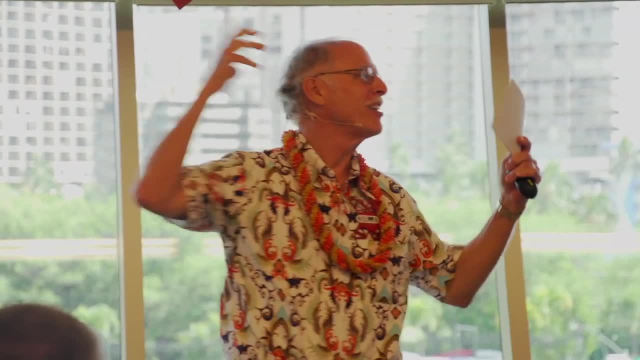 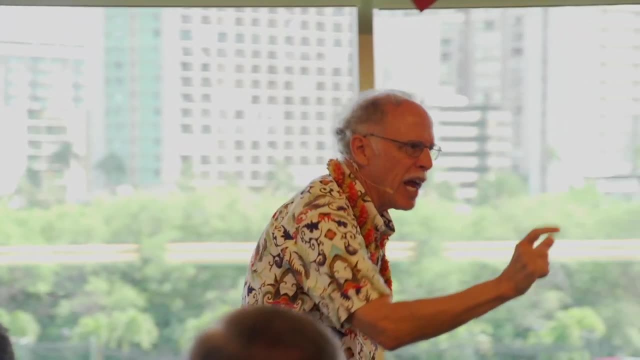 this thing is really rude, isn't it? I get really- no, I get really wound up. we get in a circle. the beauty of a circle is you get to look at everybody in the eye. you see everybody, not just the backs of heads. it was a blow to go from kindergarten. 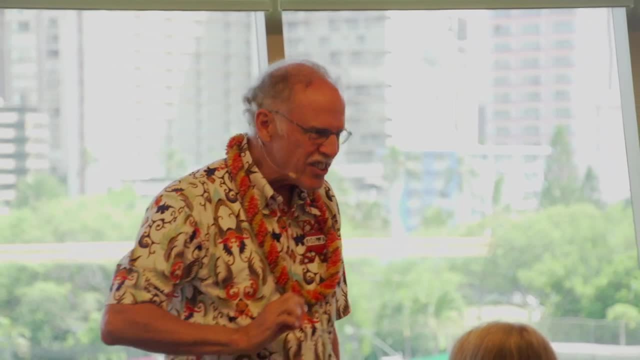 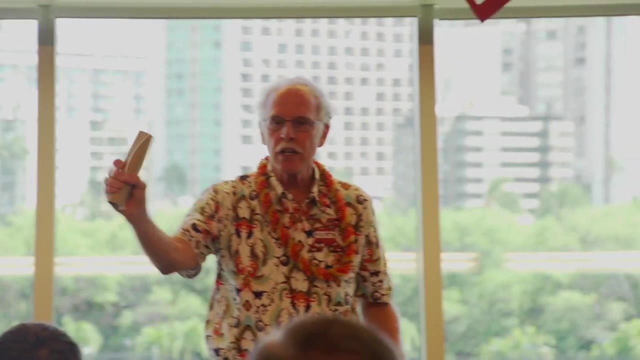 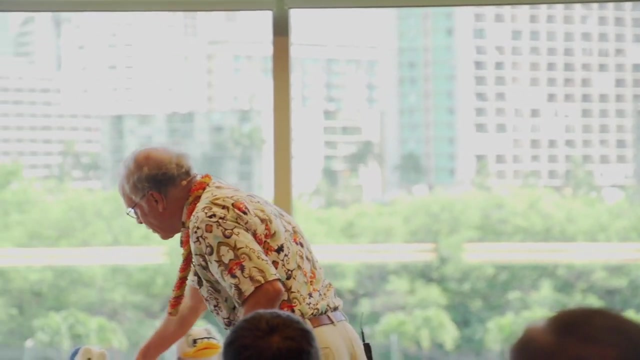 where we got to sit in a circle to first grade where all I saw was the backs of heads. backs of heads are boring. so what we do every first thing: we take something like this and something like this and we sit in a circle and we turn it into. 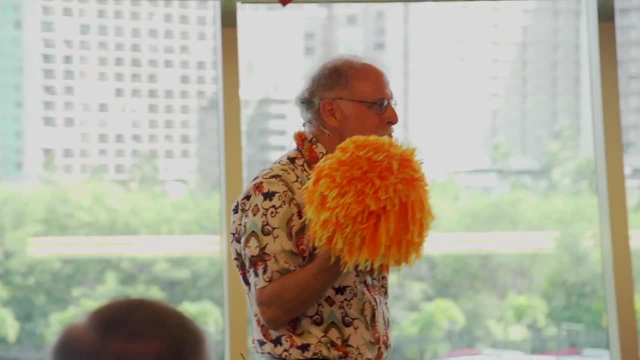 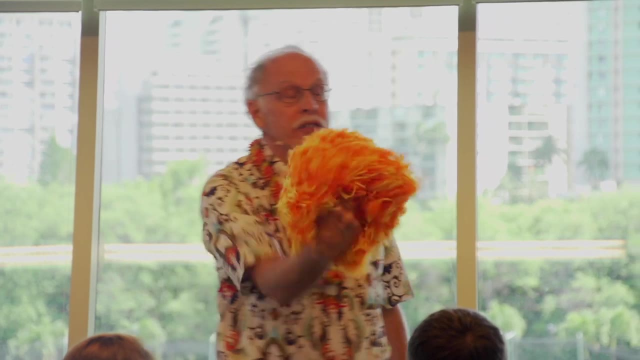 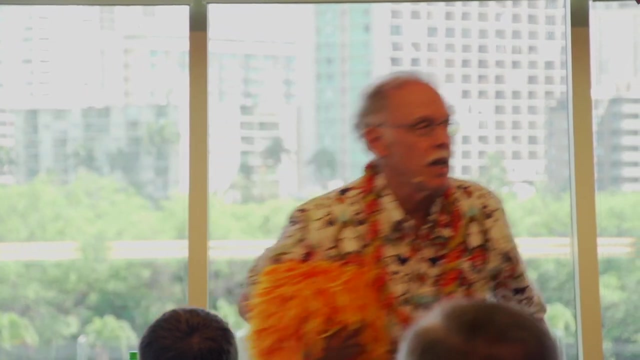 one of these. this is a community wall and at the end of this process, we're all in a circle and each whoever has the community wall, they're the one that's empowered to speak. they're the ones with empowered to speak. think of that when I think about. 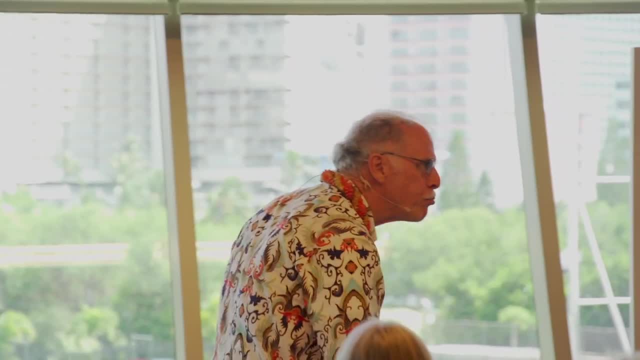 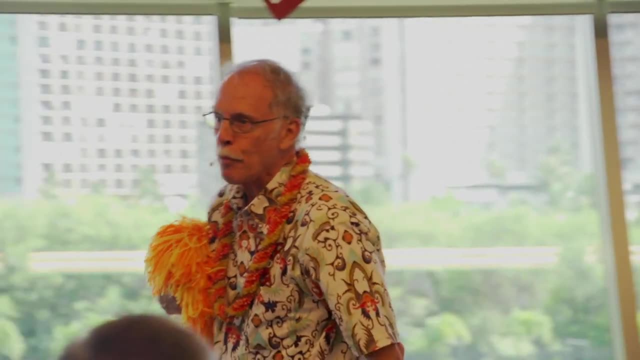 what would be an innovation in education. think about handing the power over to speak from the teacher, who has to carry most of the responsibility for that, to the individual children. and wow, do they really appreciate that? the only other thing that governs the use of this is 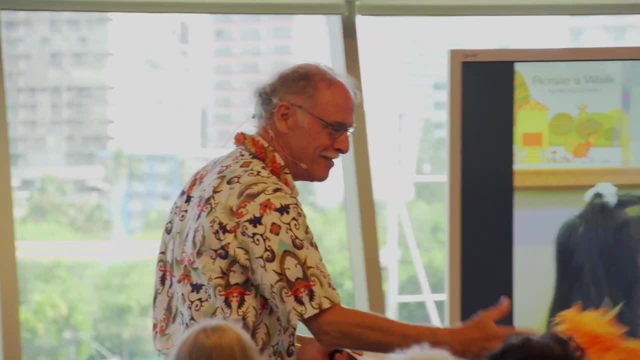 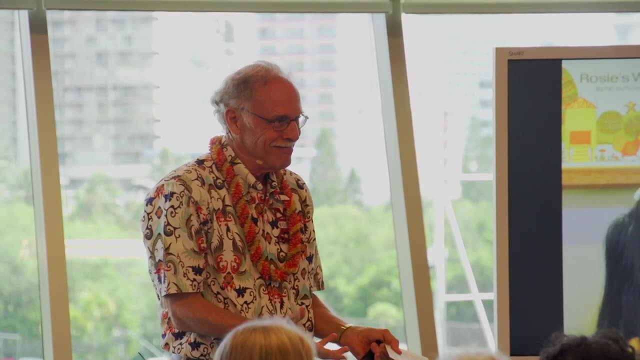 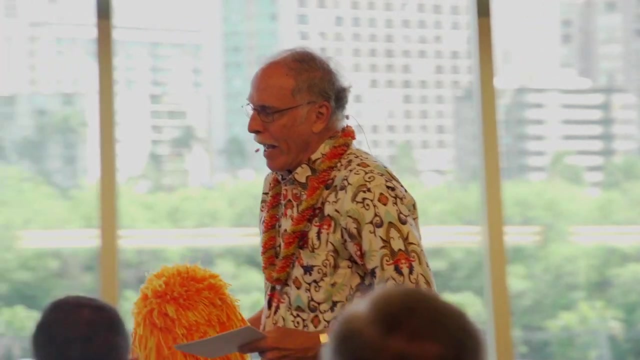 if it comes to you and if I toss this to you, if you want, you can pass. if you didn't want to, you could say: I got it now, no, and you could talk okay. so imagine, now we're in a circle, I'm in a circle with kindergartners. 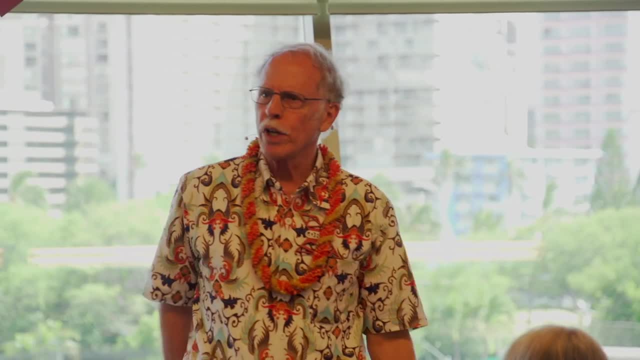 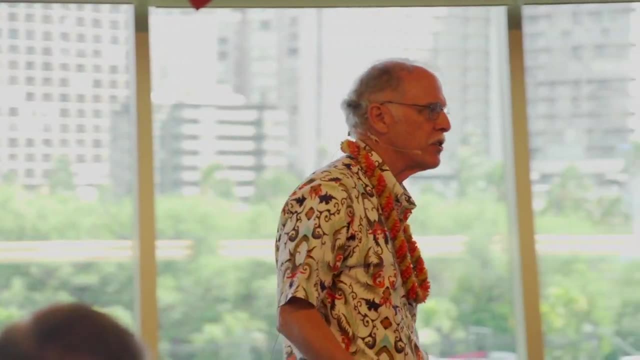 and we do a thing about finding out what the questions are that come from the children, and I think that's another incredible, incredible innovation in P4C. it's not like we don't ask for questions from kids, but when we're doing it, it's: what do you wonder about? 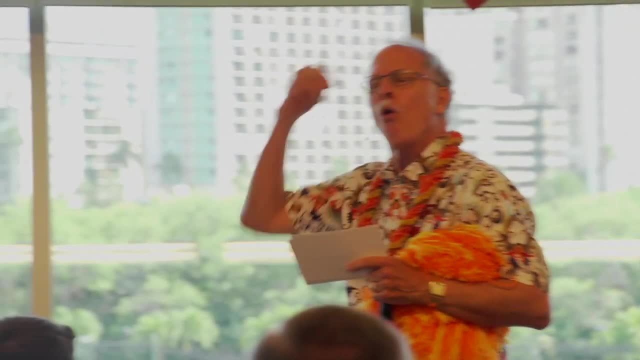 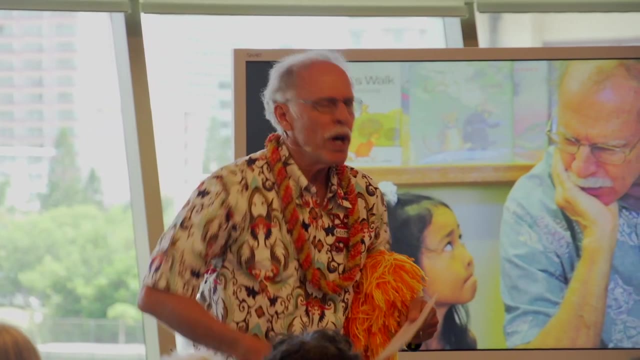 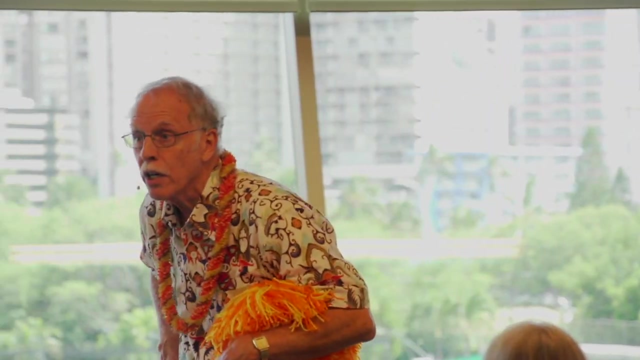 it's not a content specific thing, it's what do you really wonder about? so we pass the thing around and the kids said different things. we remember what they are. and one of the kids said: you know what I wonder about the other day when I was gazing at the stars. 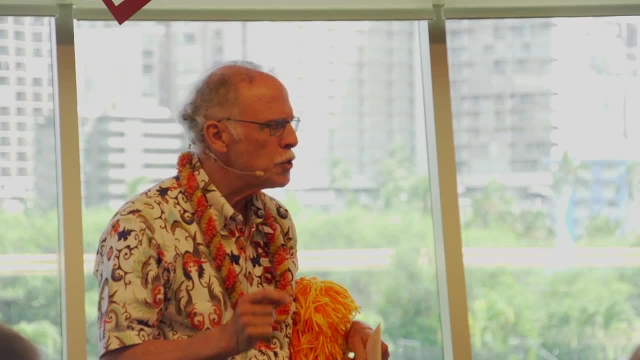 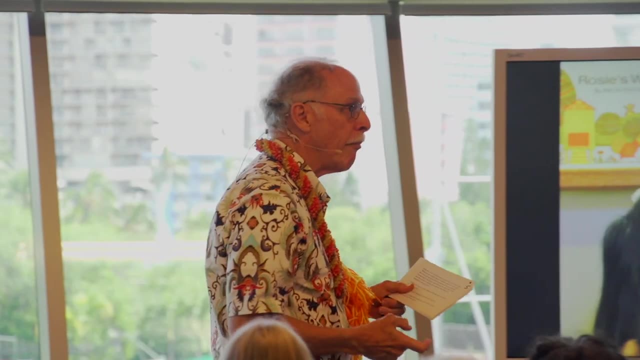 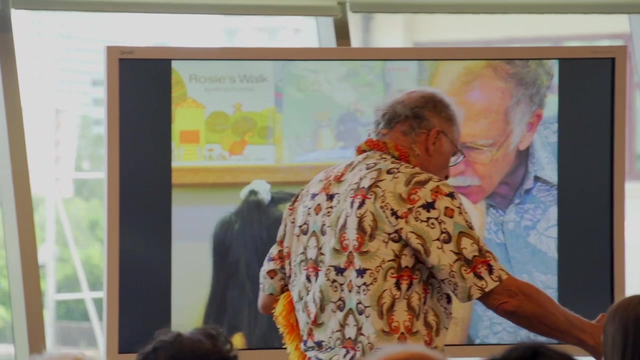 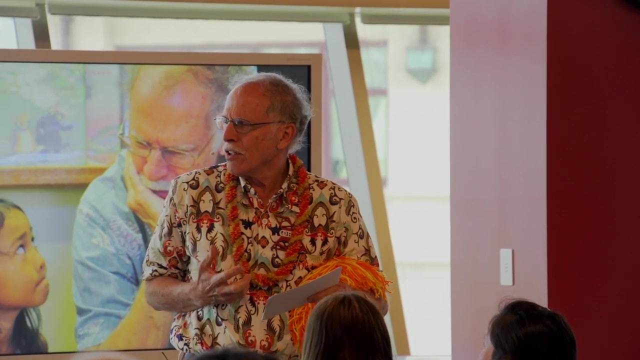 I wondered if anything came before space. did anything come before space? I'm going to give you a moment. think in your own mind, supposing this child comes up to you and says: mom, dad, where's our scientists? did anything come before space? wow, that's a wow question. 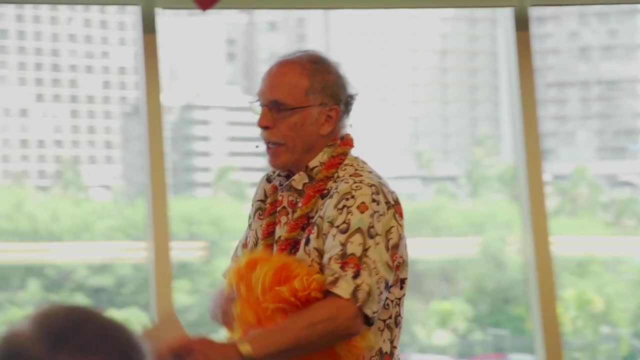 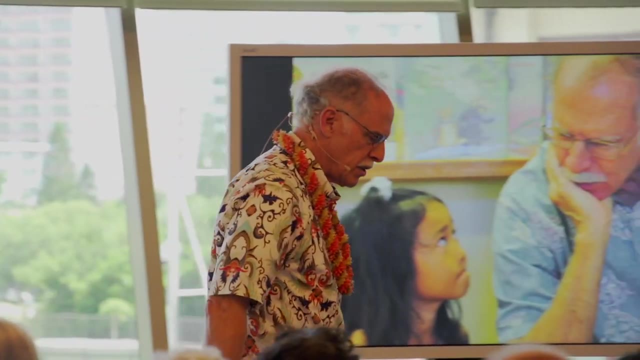 that's what they picked, and so it went to the child who asked the question and he's sitting there for a little bit- because they get to start if they pick your question- and finally he says, hmm, can I ask anybody else? he's got it and the hand goes up. 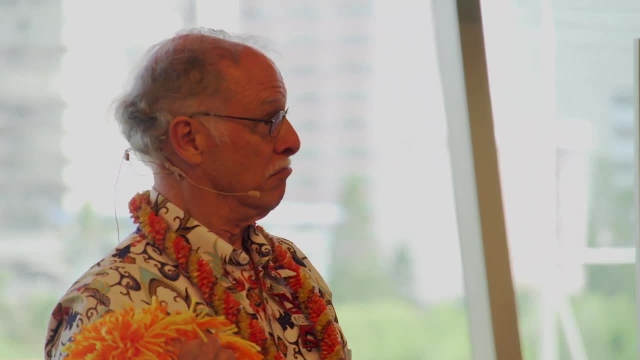 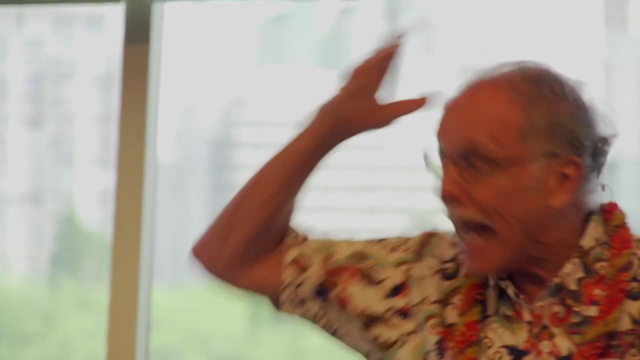 goes over to this child and he says: dinosaurs, maybe dinosaurs came before space. now I got to insert this. when you're doing this with any, whatever age, you don't know where it is, you don't know where it's going to go, and the most beautiful thing is when. 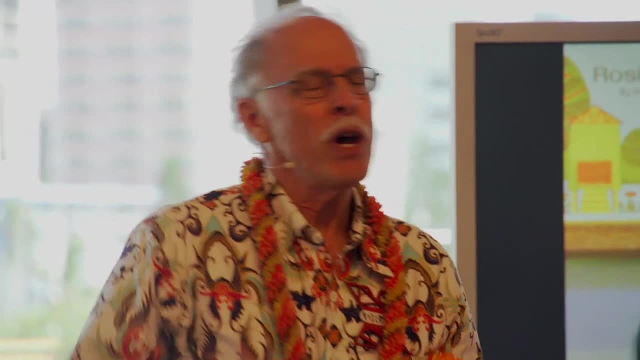 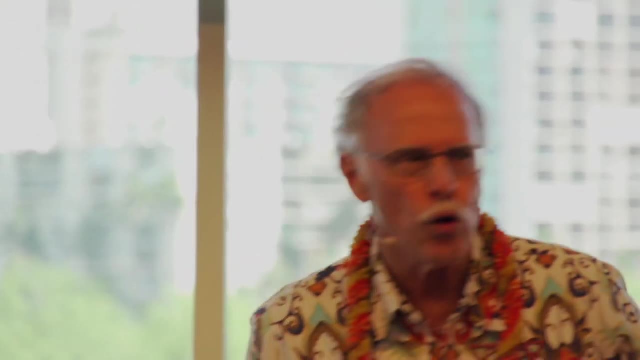 you really don't know either. you got some ideas and you want to find out what the kids think. and they get it that. you're really interested. you're not being clever and waiting for someone to come up with the right answer. no, you really want to know what they think. 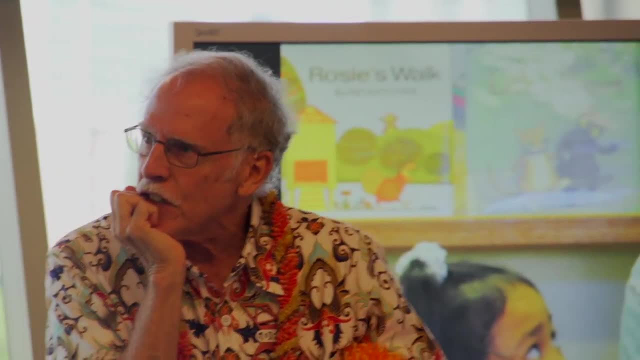 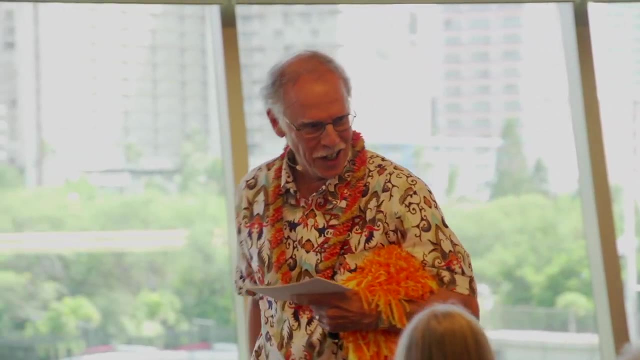 so I'm thinking wow, and I you know. so I said you know, boys and girls, help me understand what a dinosaur is. what do they have to do with space? and one kid laughs and says: space, great. now you know it's humorous, but I think when you 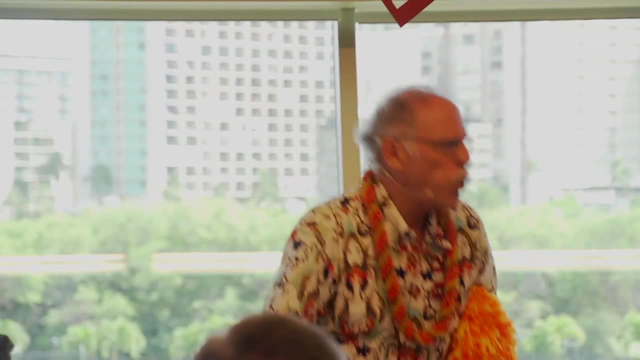 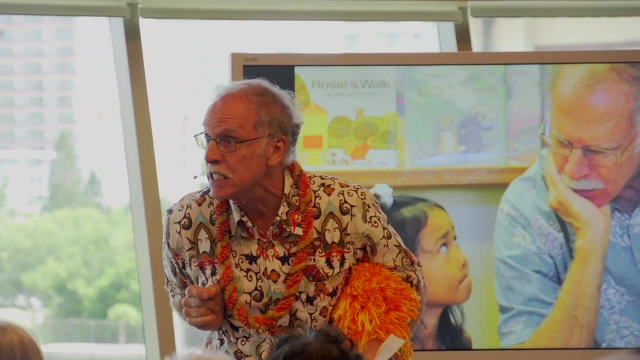 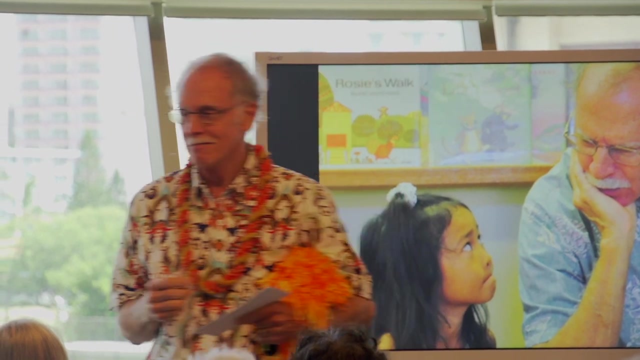 when I think of the creative thought that comes out of young children. yeah, they do. it was quiet for a couple minutes and then one child said: you know something, if dinosaurs need space, then they couldn't come before space. sometimes I laugh, laughing and say: sometimes in the early days. 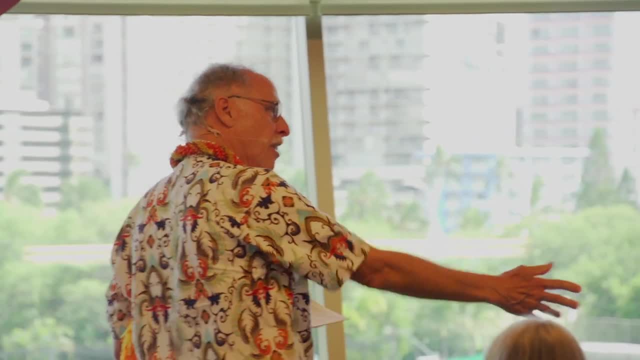 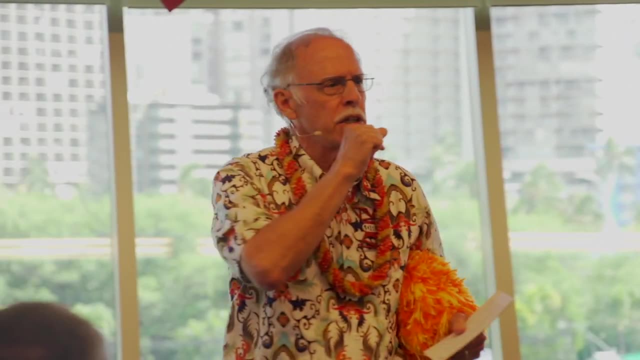 the teachers would pass out. that kid never talked. I mean, he's a bloody genius, that's really amazing. so it was quiet for a little while longer and then finally, one of the kids said: God, maybe God came before space. God is fascinating to very young children, so now it's time for lunch. 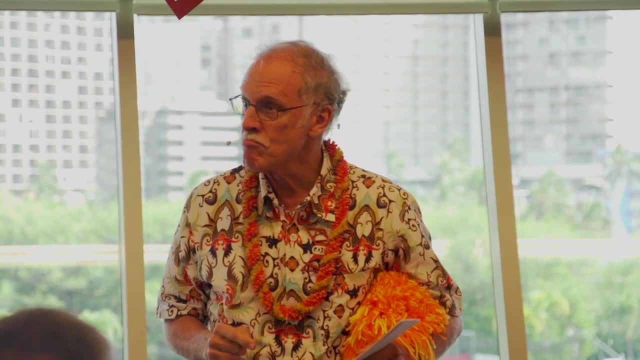 and one of the things about P4C time that's kind of irritating. that I love is the kids will say: oh, do we have to stop? you're going to lunch? no, we want to keep doing P4C. man, this is the best. this is the best. 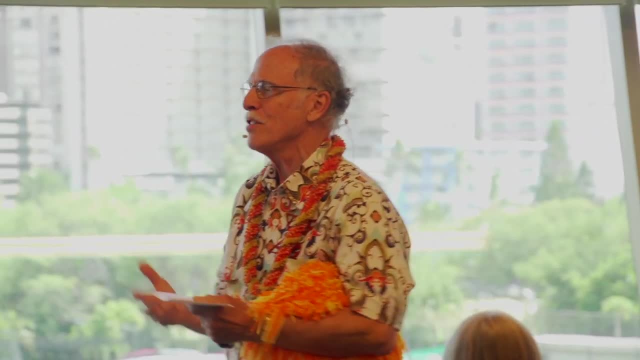 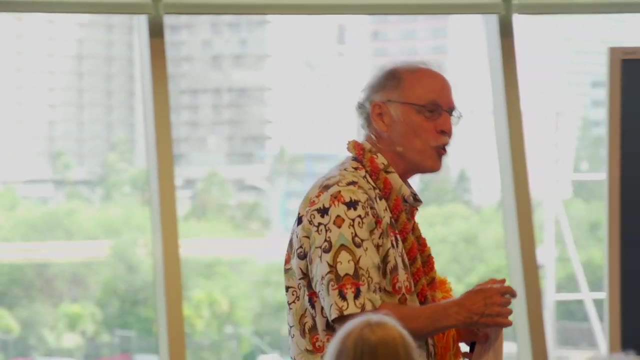 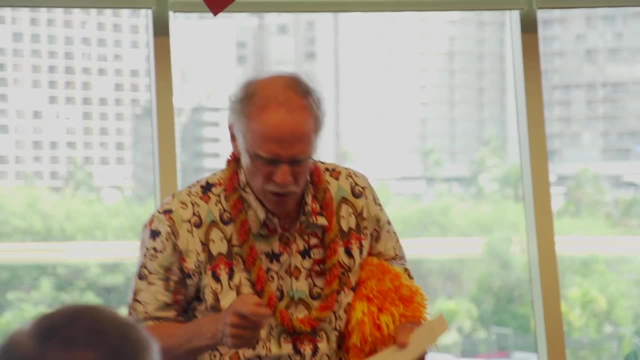 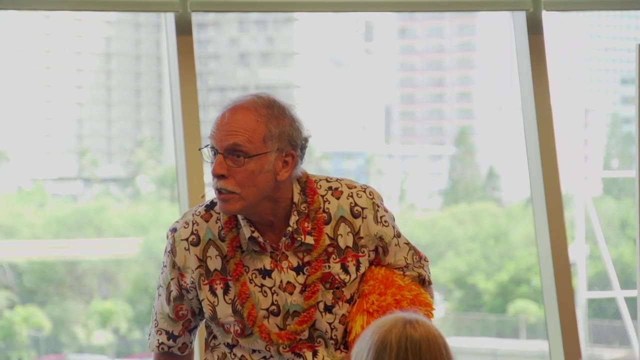 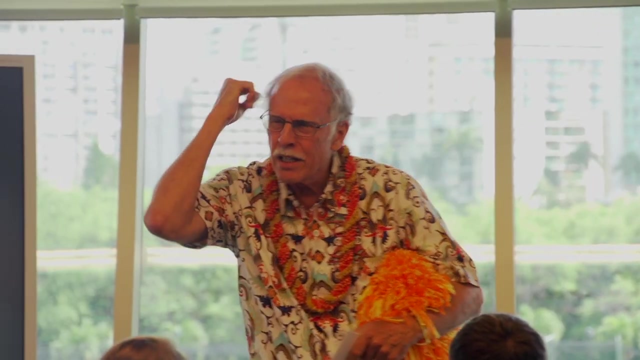 and this one of the girls comes up to me and she goes: Dr J, Dr J. you know what I wonder about. who made God? I mean, that's what happens now. I was going to make what are we two minutes? wow, we're two minutes, ok. 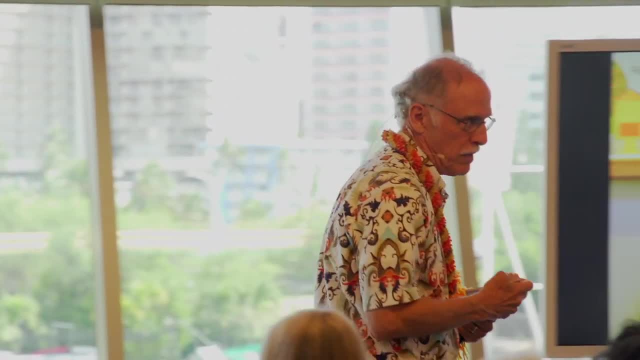 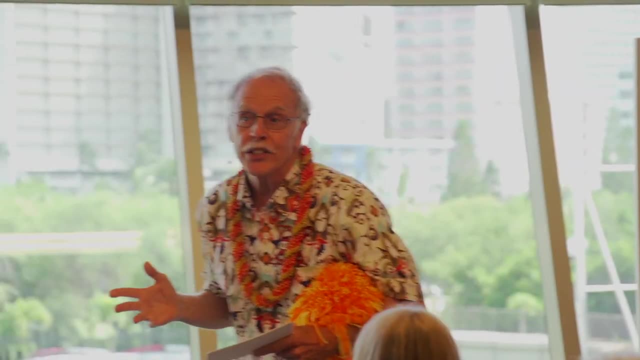 so I figured that in this time I could only give you a little taste of this. there's some schools on the island here where they're doing P4C. they've been doing it. Waikiki Elementary has been doing it for about 14 years. Kailua High School. 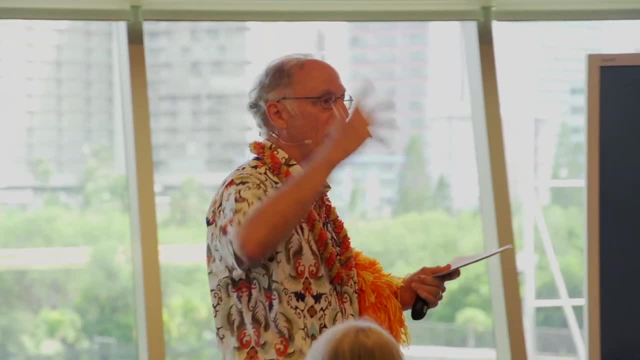 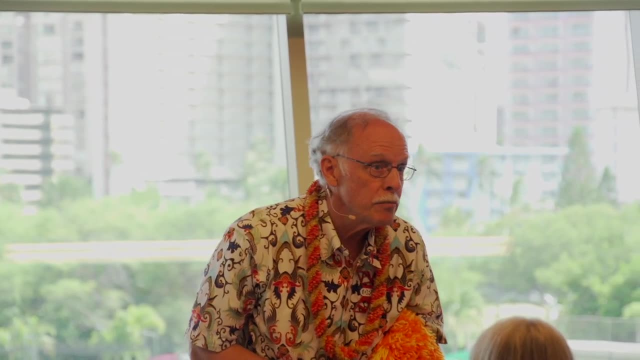 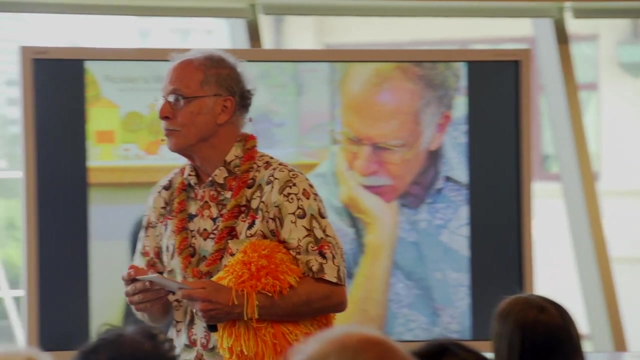 has been doing it for about 12 years. I want to sneak this in. when the Dalai Lama visited Hawaii in April, he went to Kailua High School because of the way P4C had changed the culture in the school, and and, and, and, and. 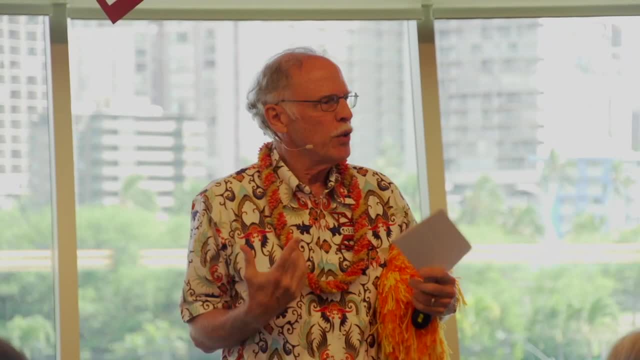 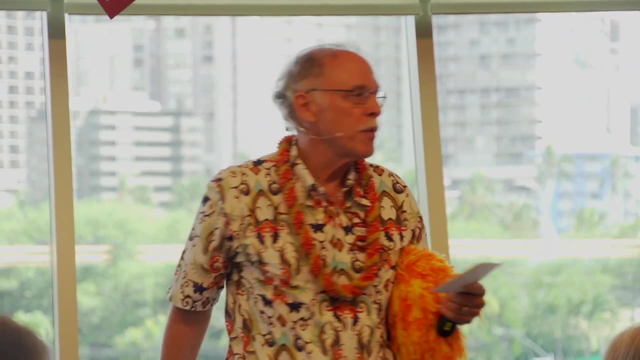 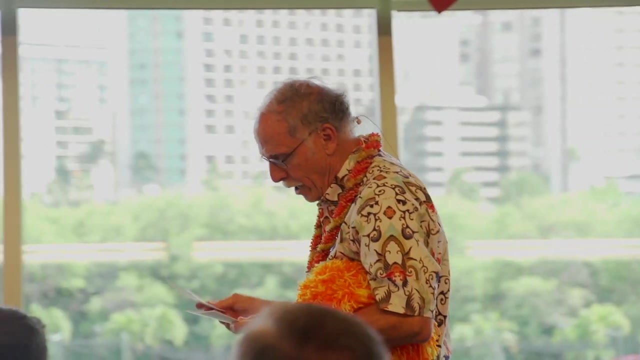 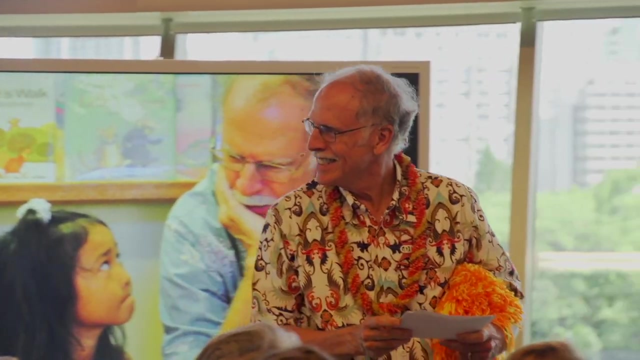 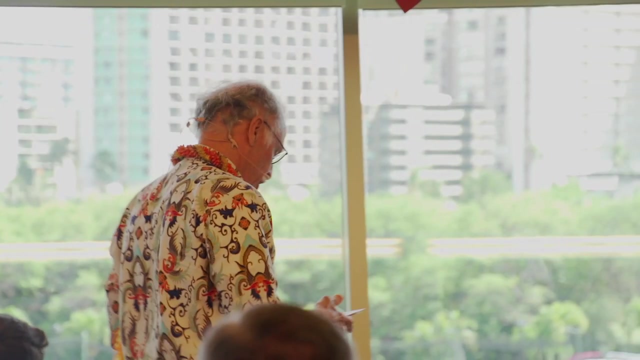 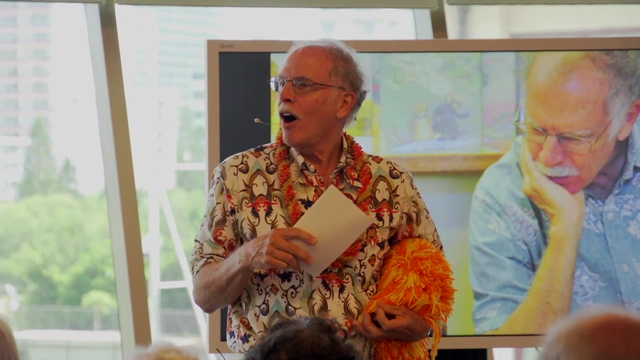 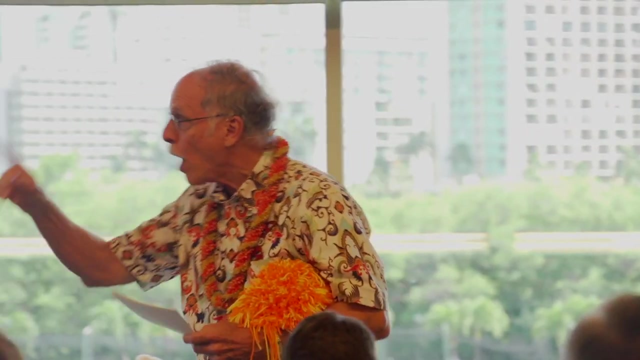 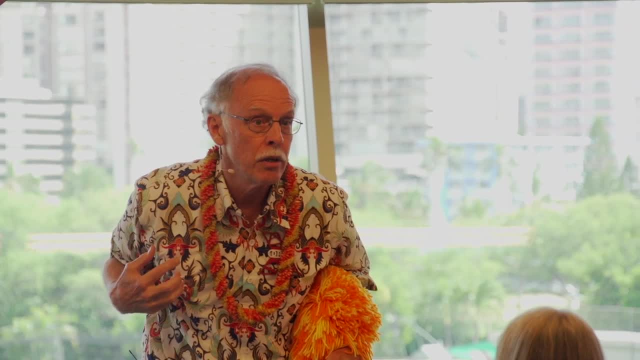 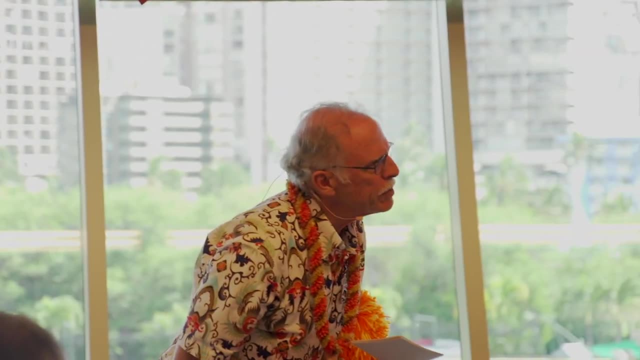 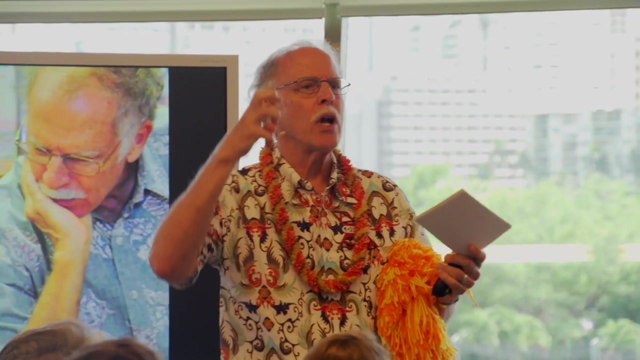 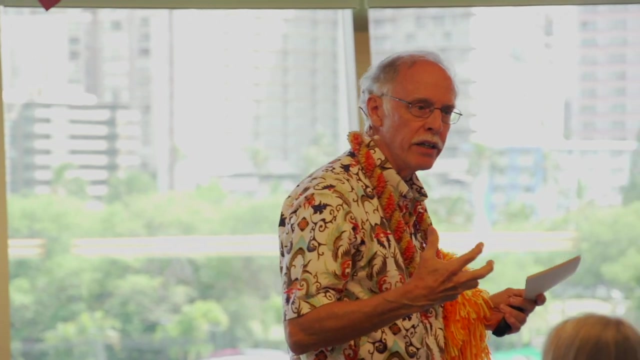 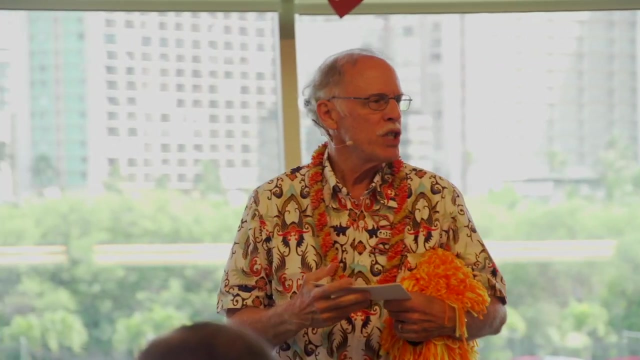 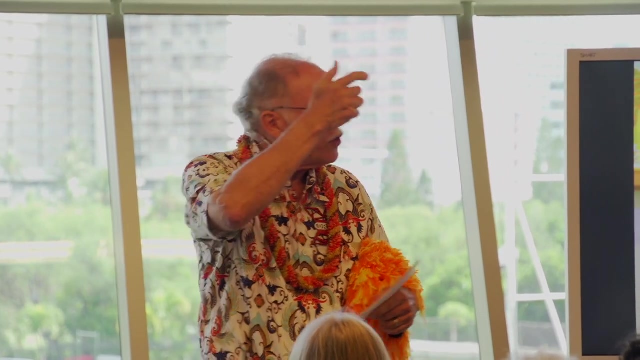 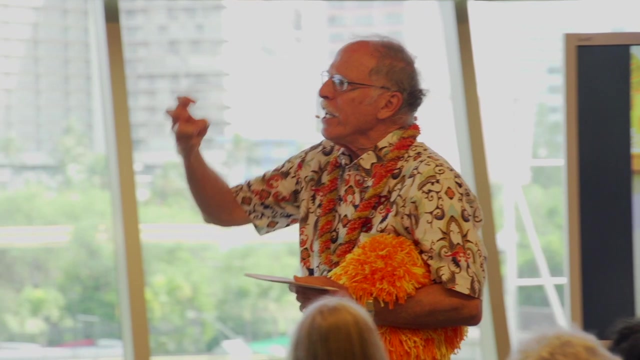 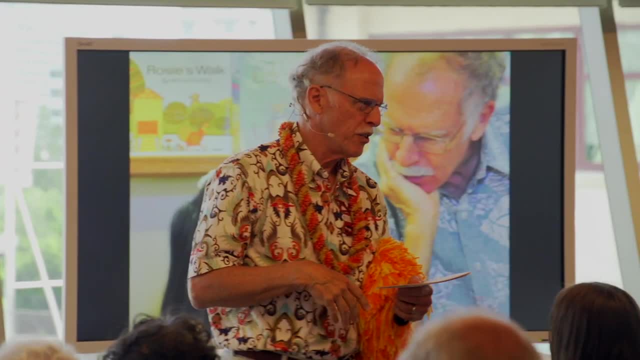 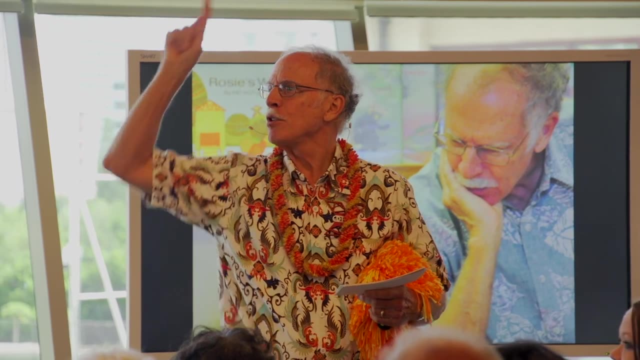 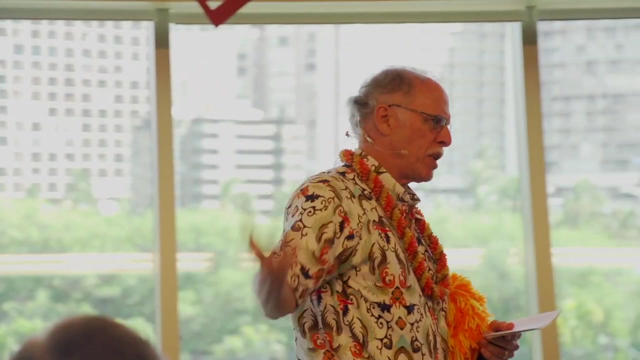 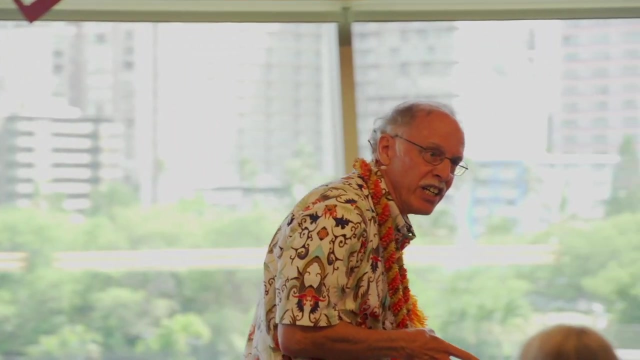 but again something one just came hitting: experience telling the well either until They're absolutely brilliant. Maybe it was a busy week last week for the truth fairy. She's behind in the schedule. Maybe she's sick, You know these kinds of things.